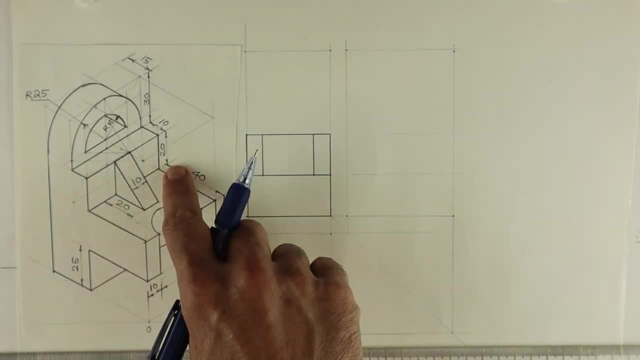 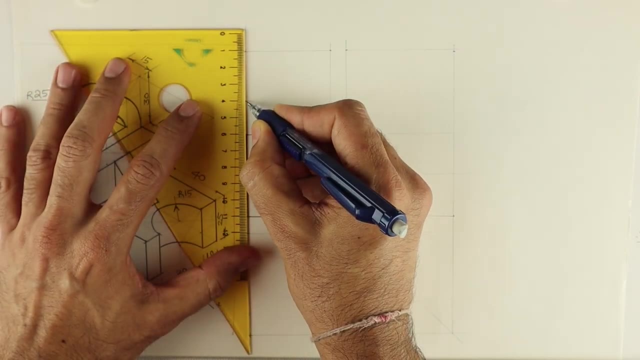 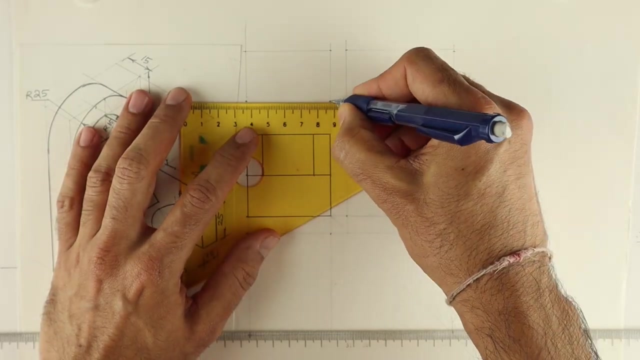 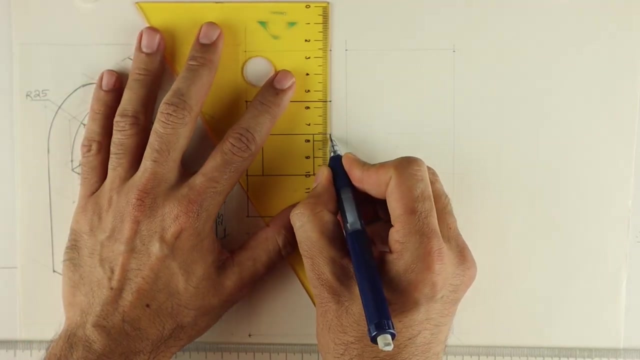 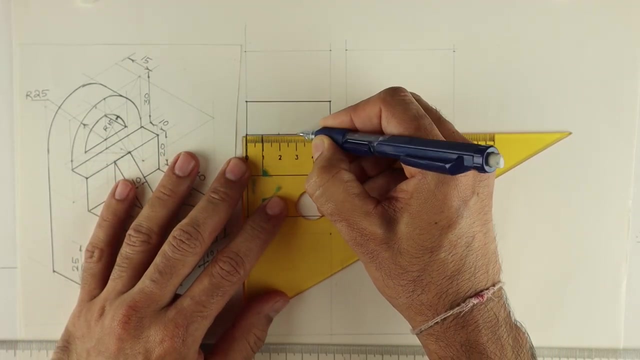 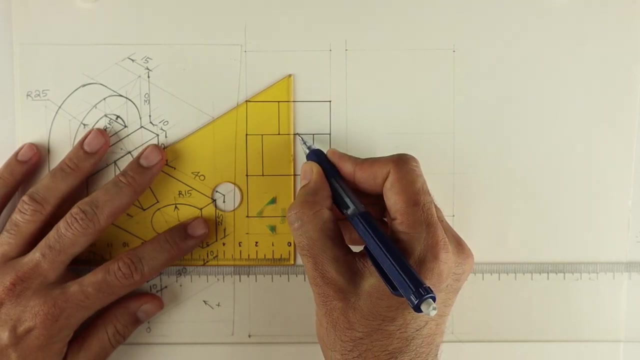 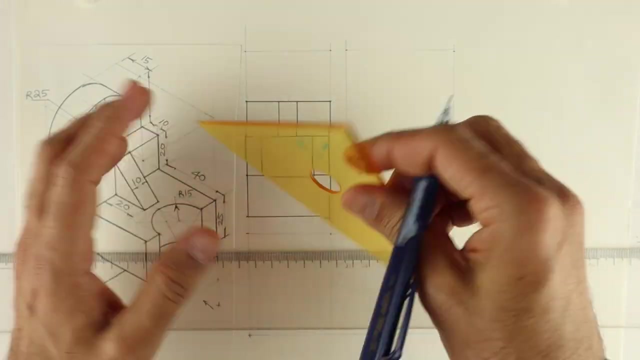 Now, after that, this part. This is 20, 10, 20.. Height is 20.. See this. So what we can do This is: I'll take 20 from here, midpoint, 10, 10.. Now, if you see, the height is 30.. 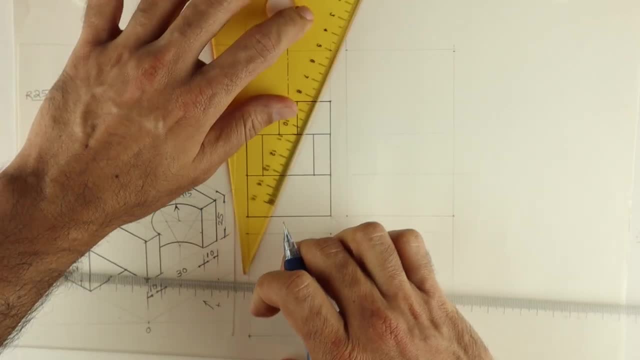 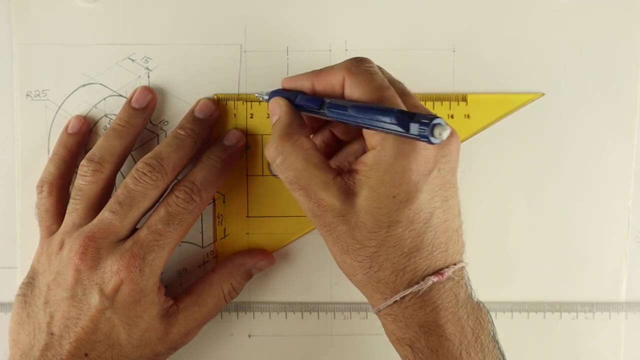 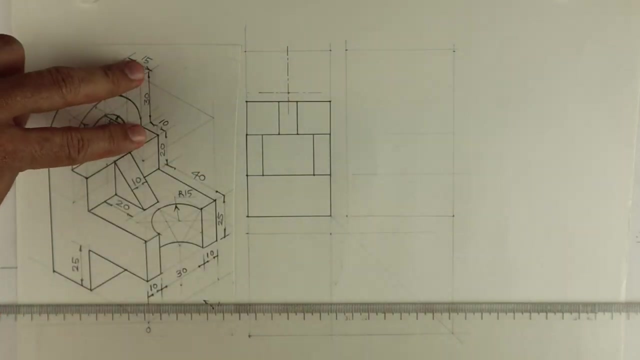 And the radius. what we need to draw is 25.. So from top we will go down by 25.. Remember there will be a 5 mm gap. So this is center line for the circle. Now this is 30. But the radius is 25.. 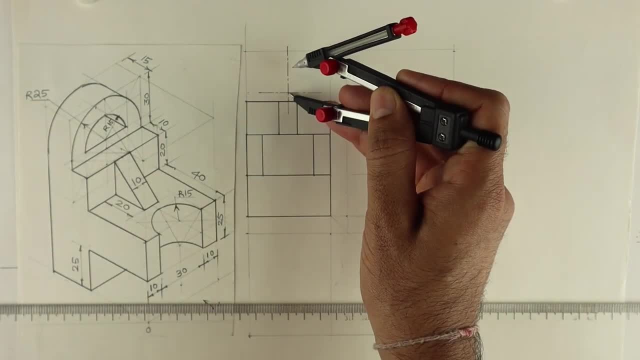 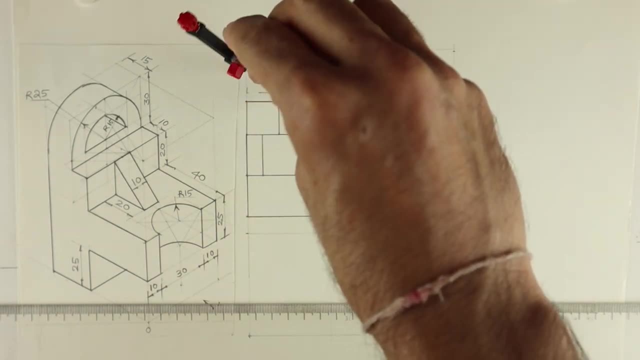 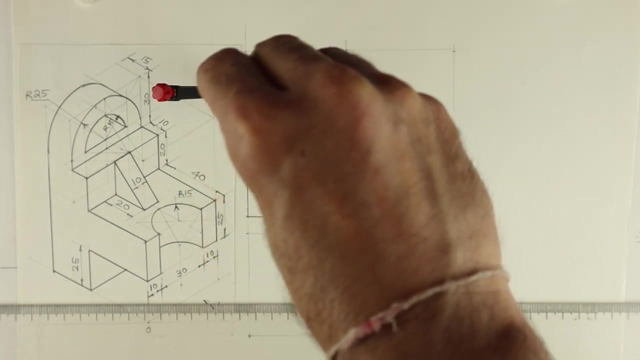 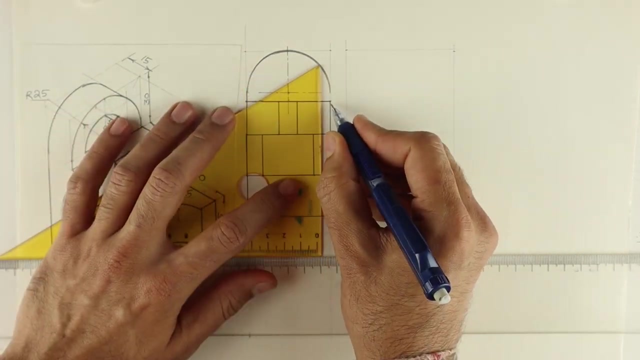 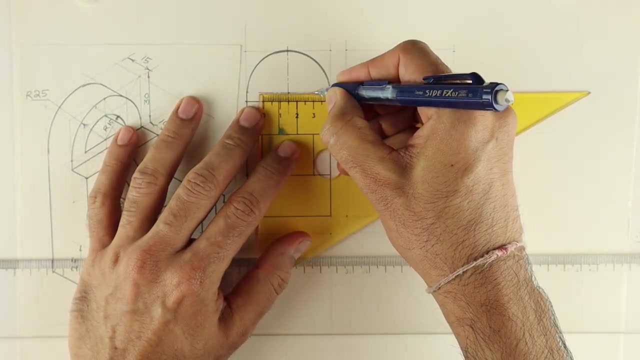 So from top you go down by 25 and you draw a circle. Now there is one more circle, of radius 15.. See, this is 5 mm, which I was talking about Now radius 15.. So from center again, you take 15, 15 on both the sides. 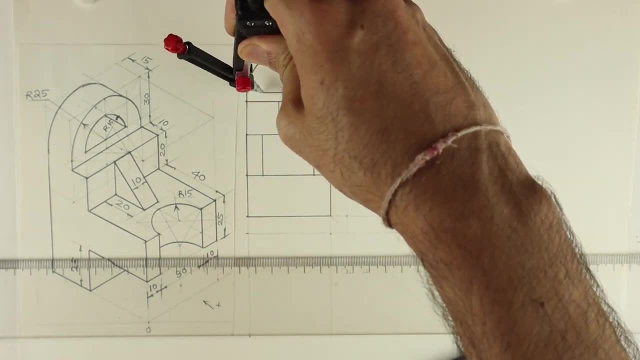 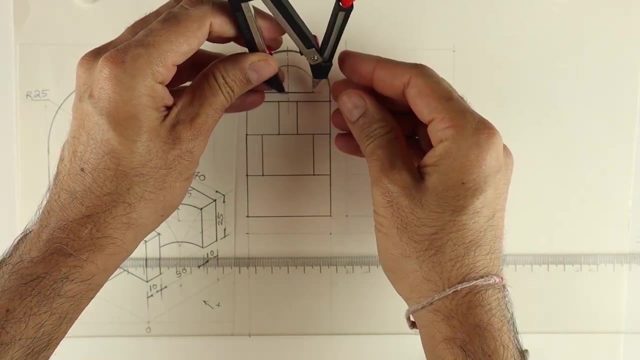 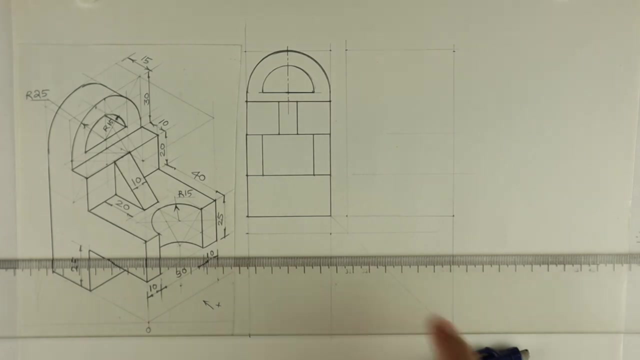 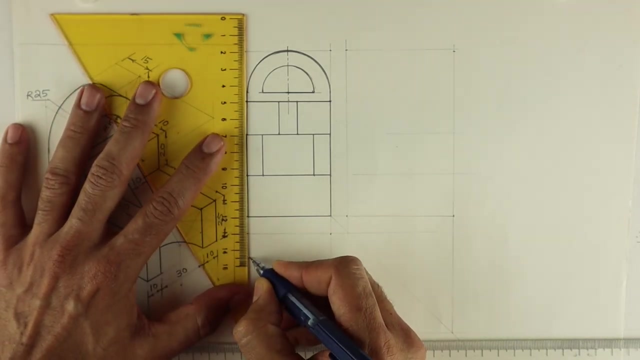 And we can draw. We can draw half circle like this. So we are done with front view. Now we can draw top view. In top view, we will see this part 15. Which will be rectangle. Always remember: circle in one view. 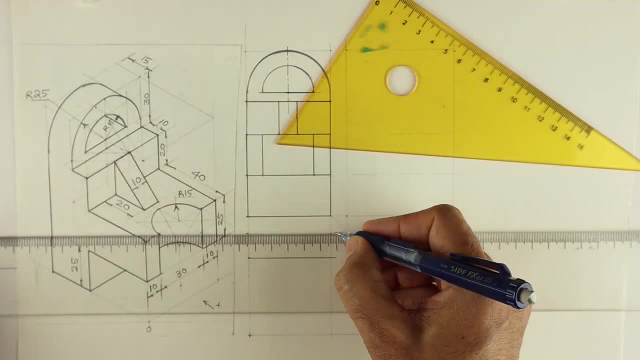 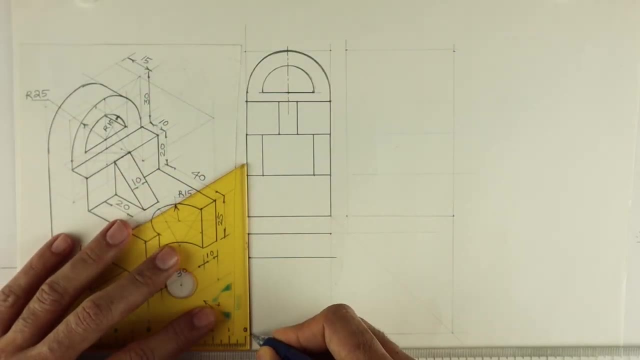 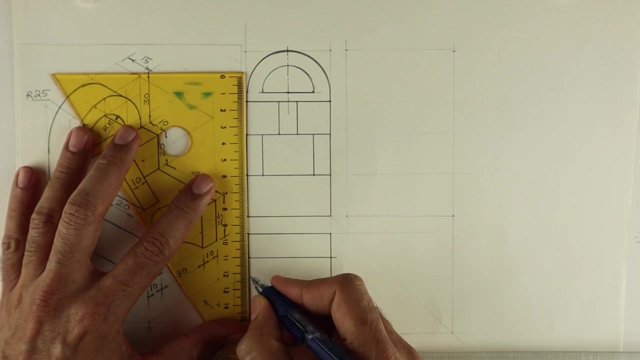 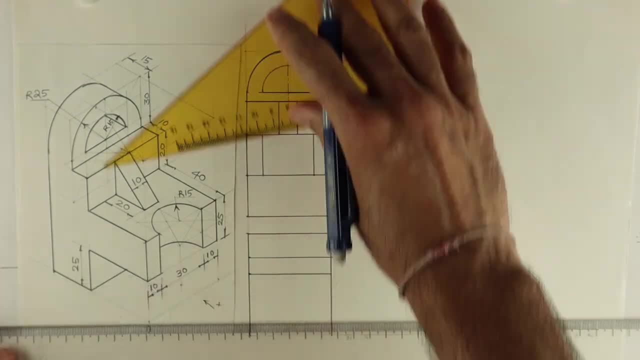 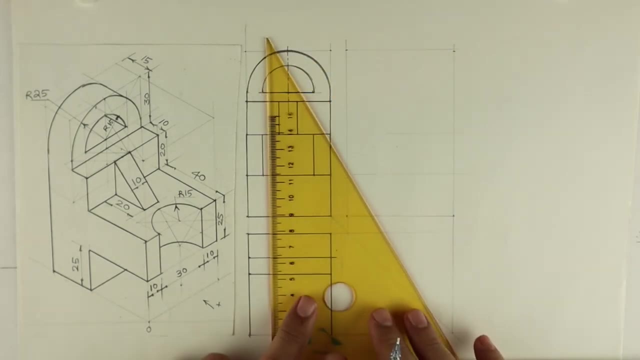 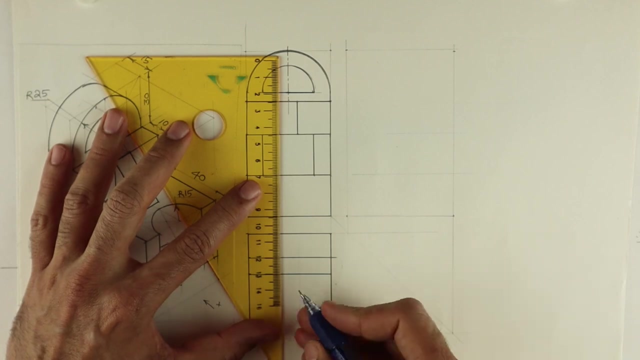 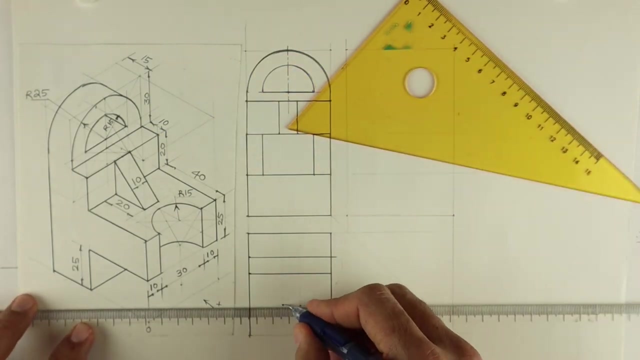 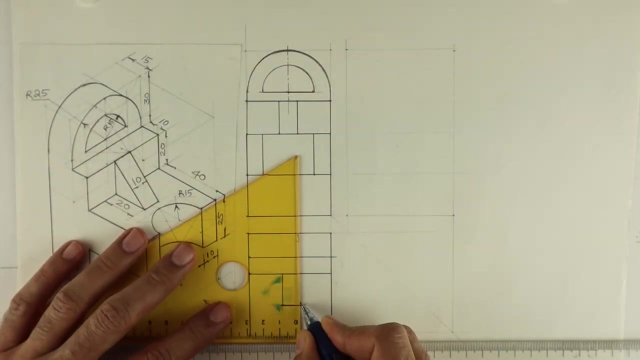 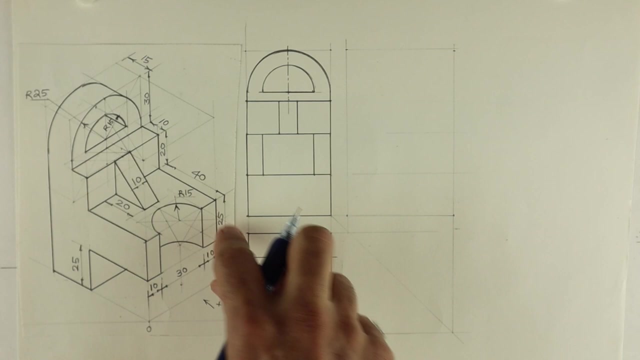 So we take 10 from here, Again you draw line, Then we have this 20.. This slope will appear as a rectangle. Now, after this, we need to draw this circle, Which is radius is 15.. So take center point and take 15,, 15 on both the sides, and again you draw half circle. 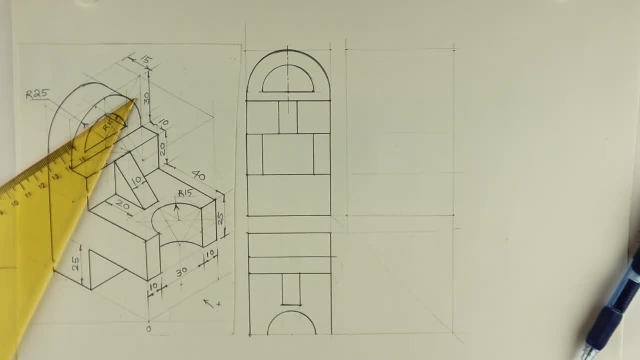 So we are almost done with top view. We need to draw dotted line in top view. This will be dark. Now for dotted line. what we need to project, LR. This is the extreme left and right of the circle. See, this is over here in front view. 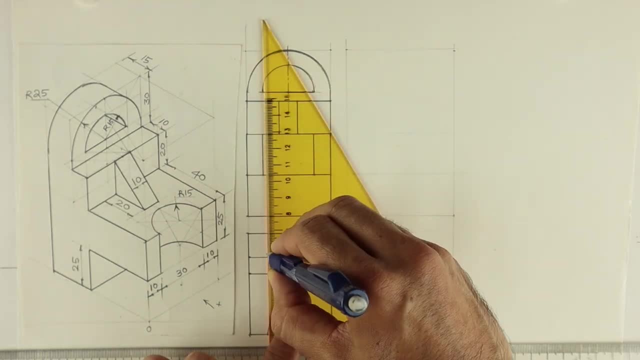 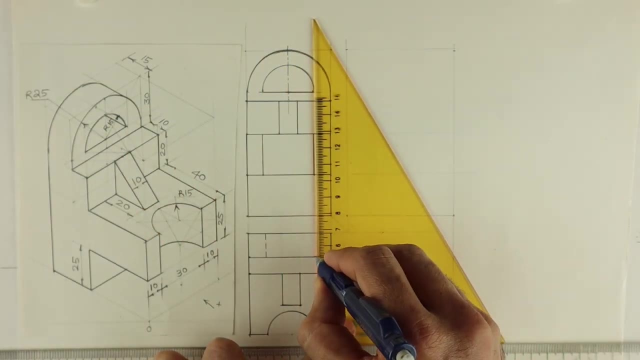 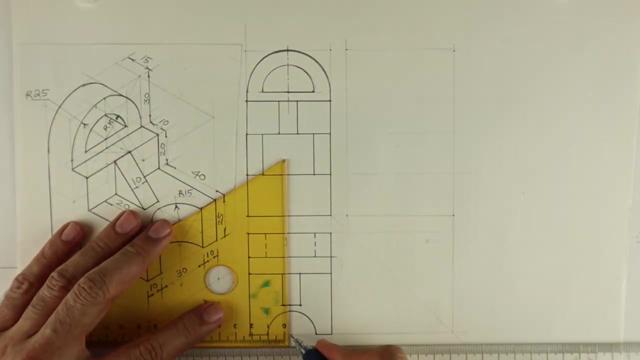 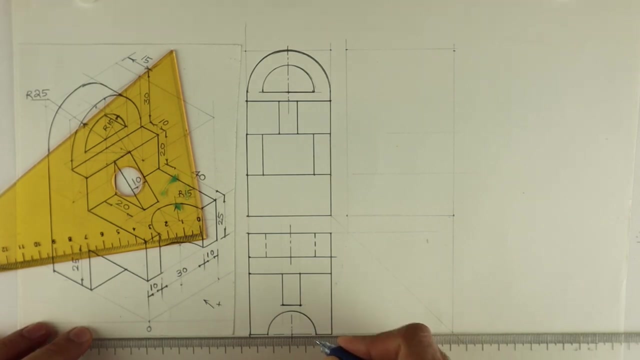 Same way from front view. when you project, it will be here. So this part we can't see, So that's why it is dotted. Always remember the part which we can't see that we need to draw dotted. This is axis. Now we will see side view. 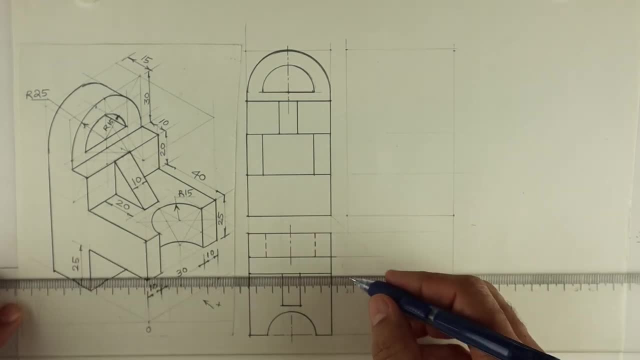 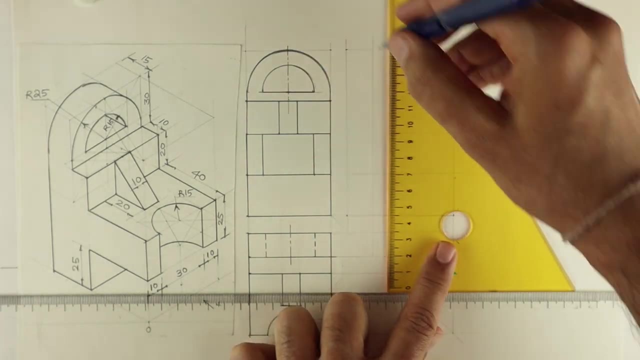 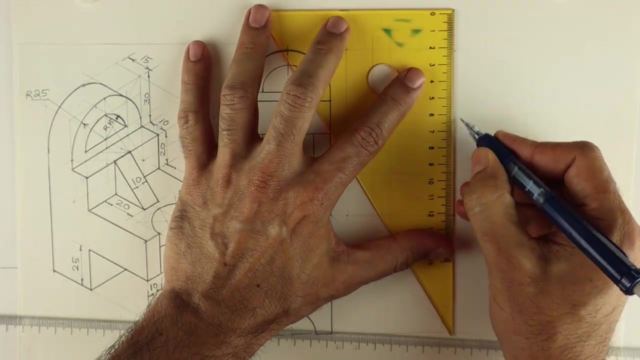 Inside view. we will start from here: 1. 1., 1., 1., 2., 1. 2., 1. 3., 1., 2., 3. 3.. ил 1.. 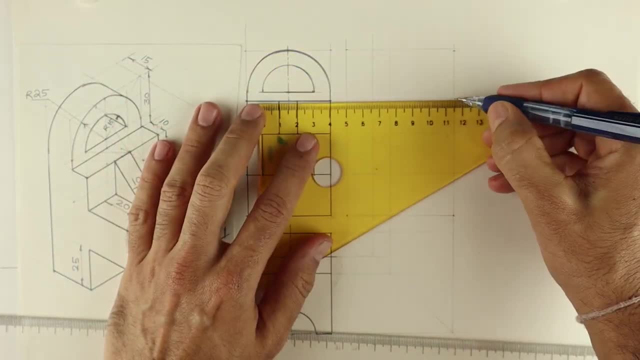 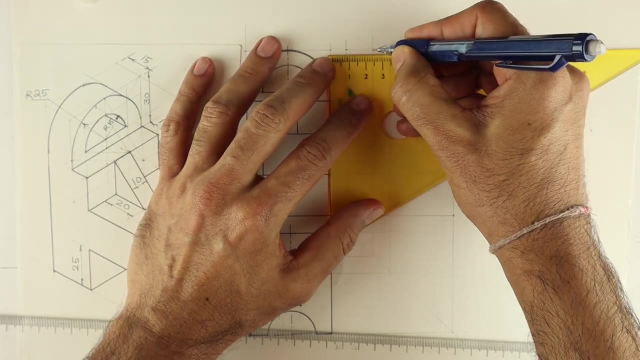 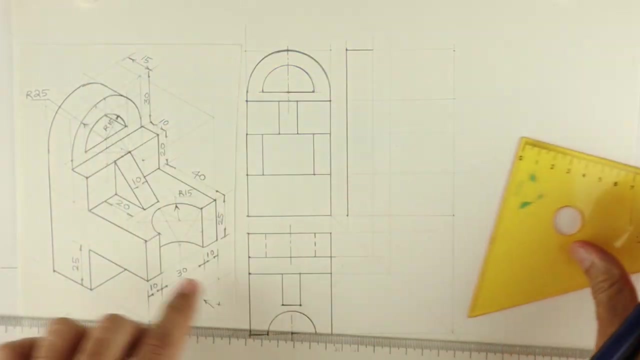 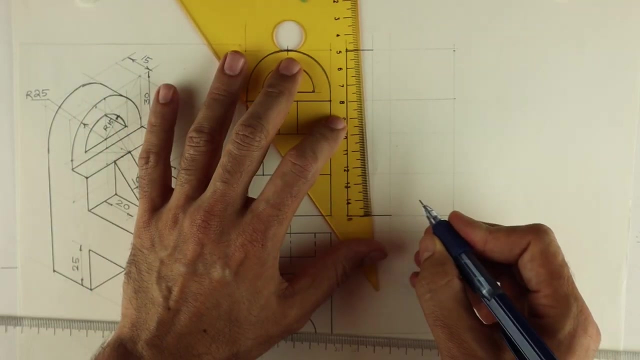 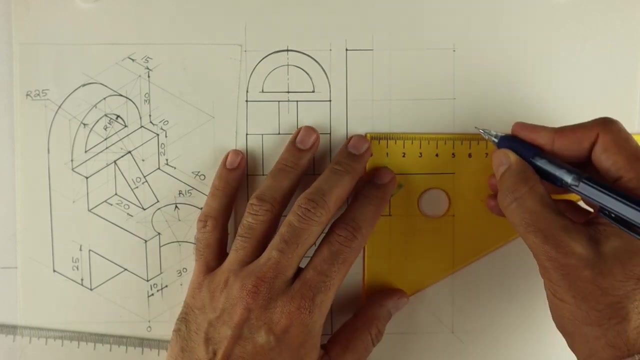 2., 2., 3., 1., 1., 6., 7., 8. part so from top 15 and go down by 30. this is straight. this is 25, 15 plus 10. then you go up by 25, then again you drop 40. 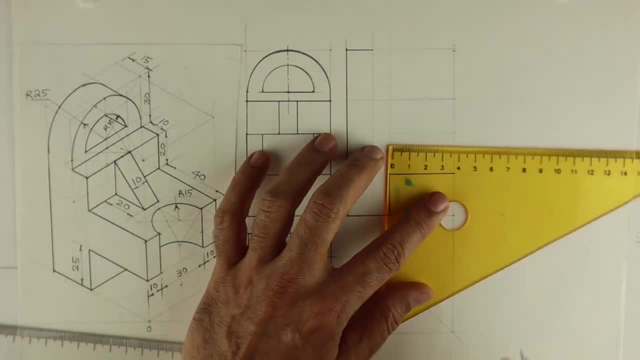 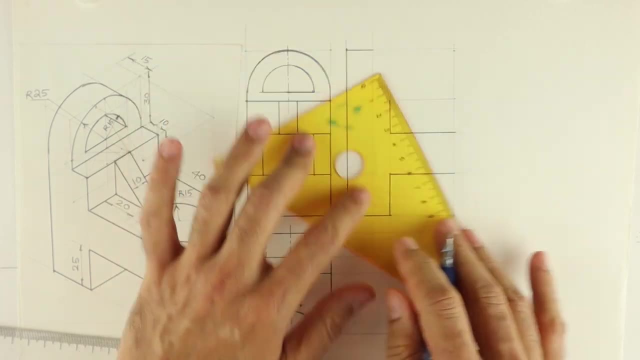 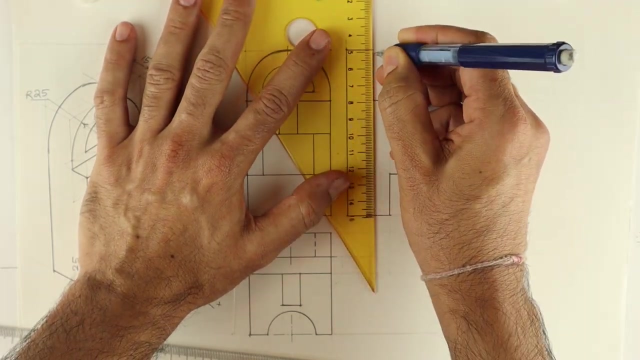 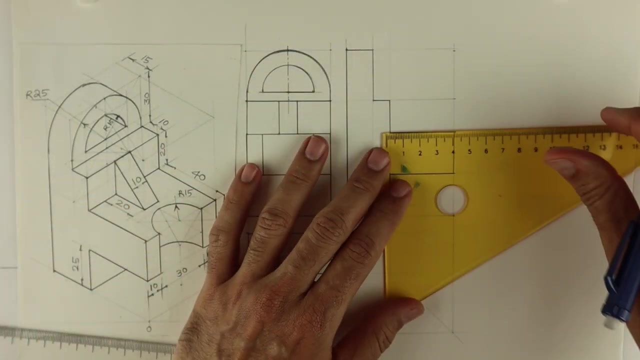 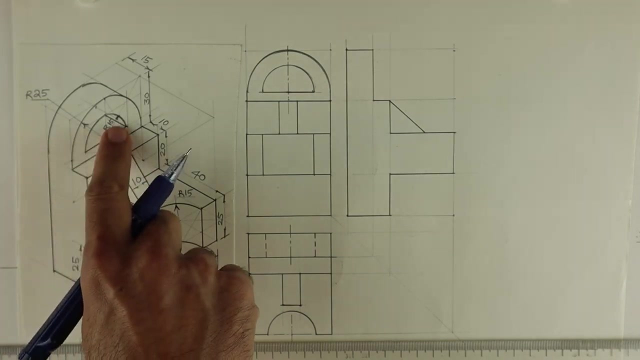 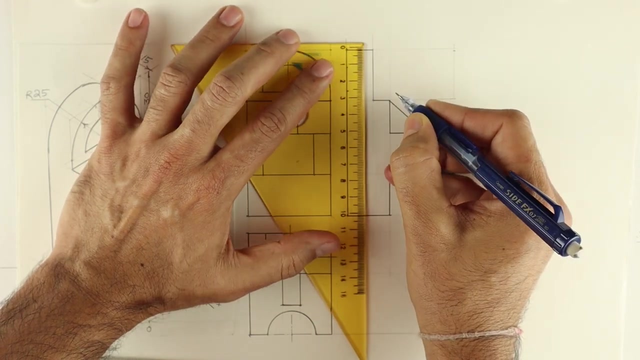 this is 40. go up. then again you draw 10. this will be dark. this is 20. so now only we have. now we have to draw only dotted line. see this part, extreme top portion and the center line. so in this we'll have two dotted line in side view. one is for this. 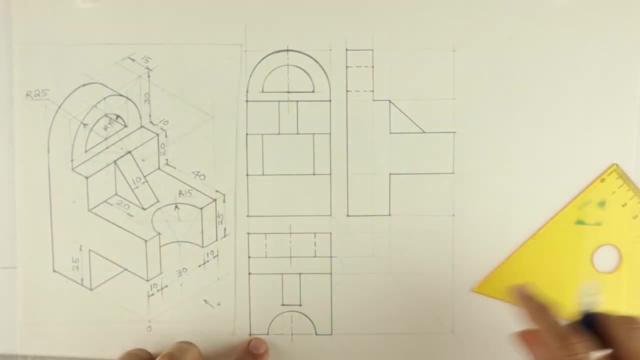 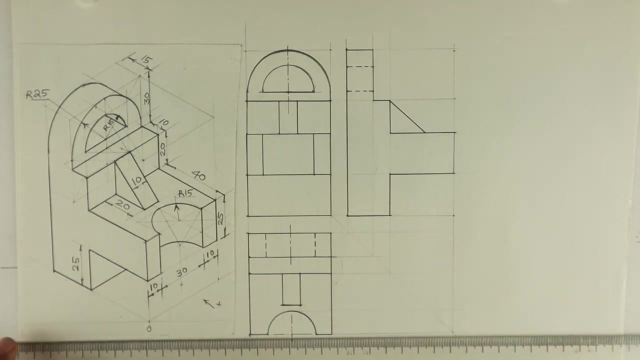 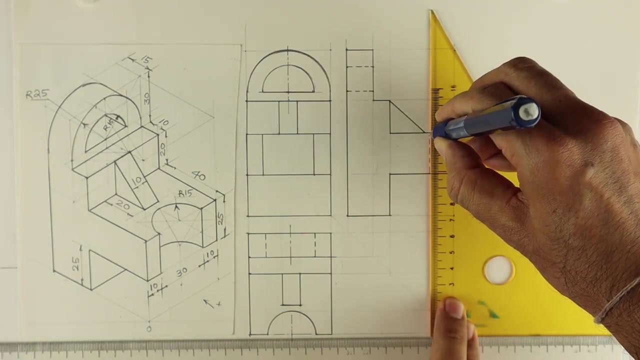 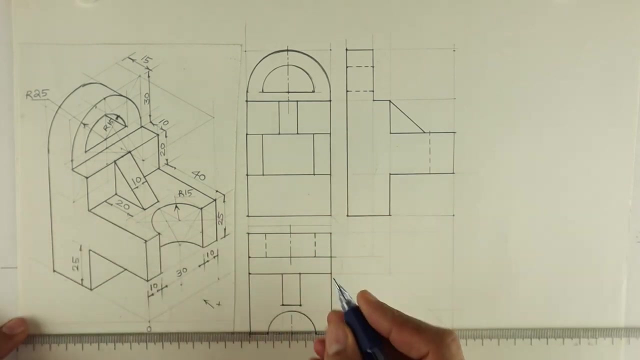 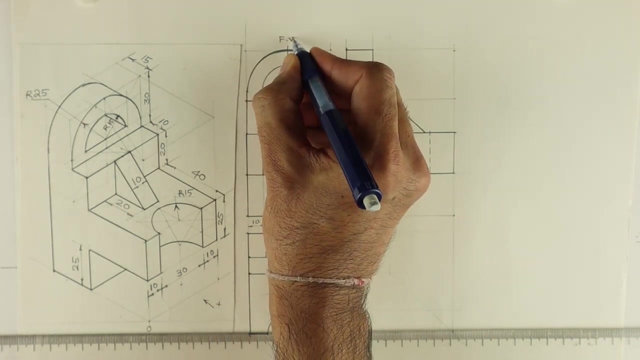 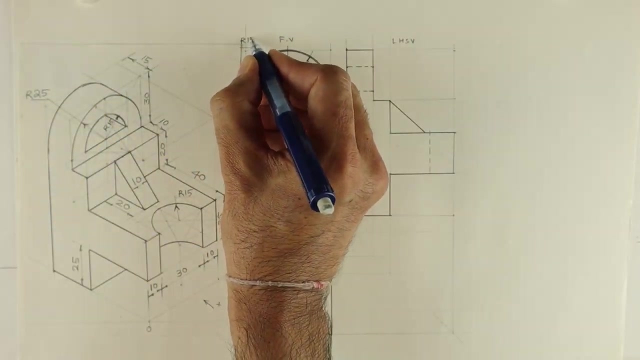 and one is for this and one more dotted line for this, that you can project from side top view. we can project from top view to side view, see like this: so now we are done with the sum, we can do labeling and dimensioning. thank you. so now we are done with the sum, we can do labeling and dimensioning. 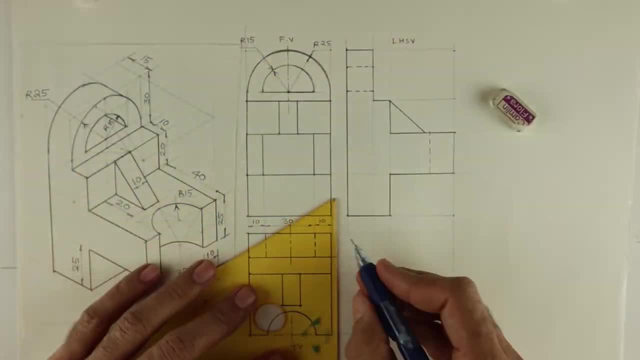 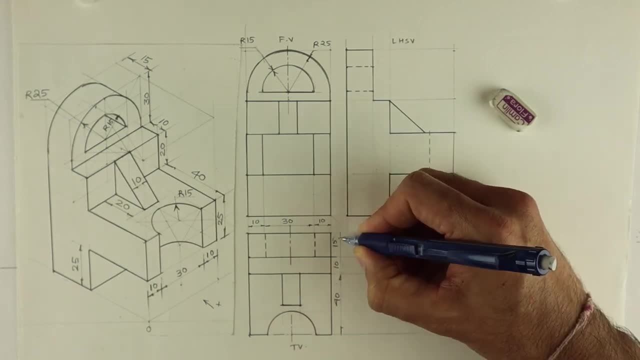 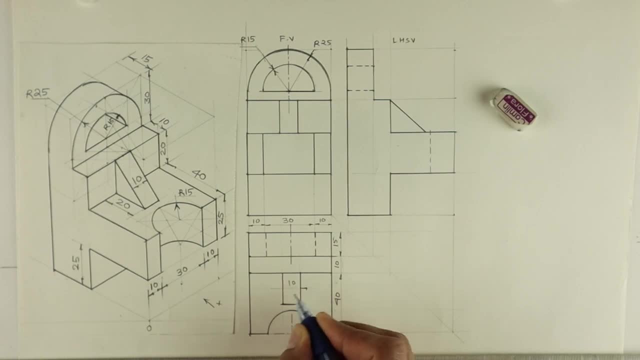 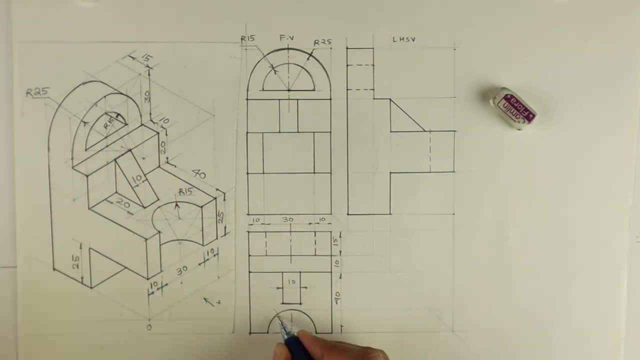 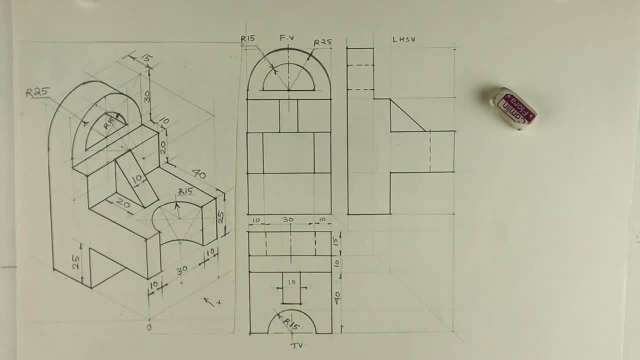 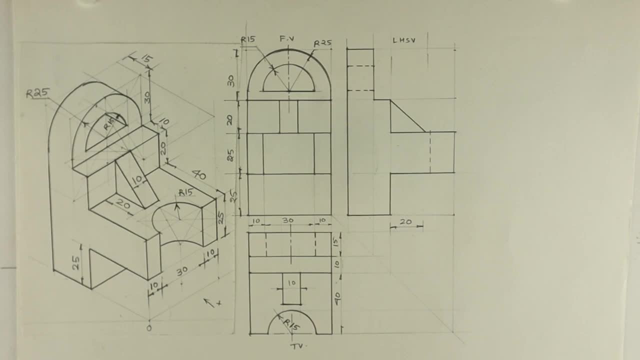 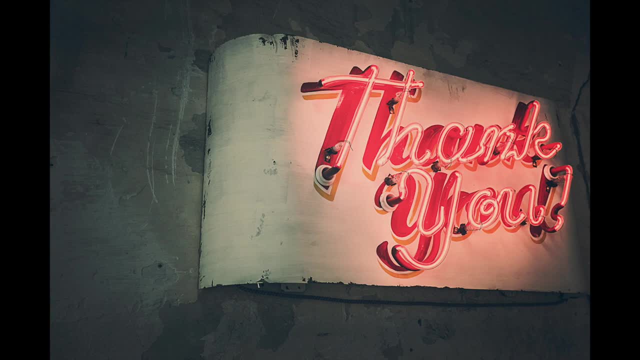